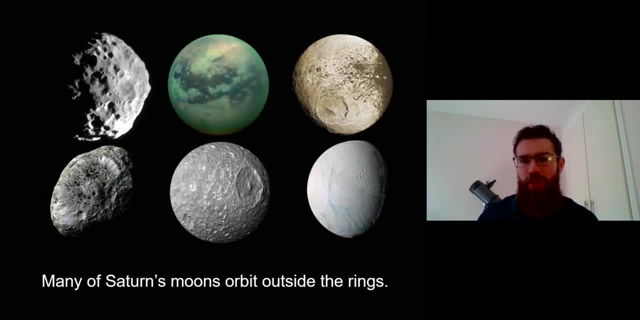 So you have all of these moons orbiting outside the rings. So you've got Titan's biggest moon, you've got Enceladus, you've got lots of different moons that are all orbiting outside of Saturn's rings, And we'll do another video to have a look at these. but these are actually causing orbital resonances that can cause a gap in the ring. 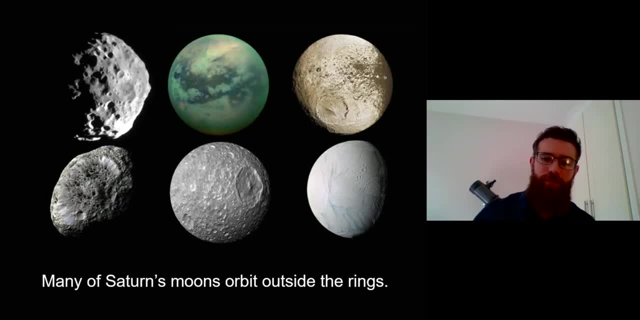 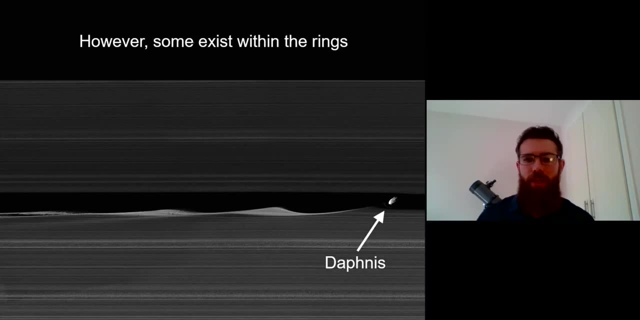 So they're all orbiting outside of the ring, But there are actually some moons that orbit with inside the rings. So, Daphnis, here is a moon is orbiting inside the ring And you can see it there. to the to the right. 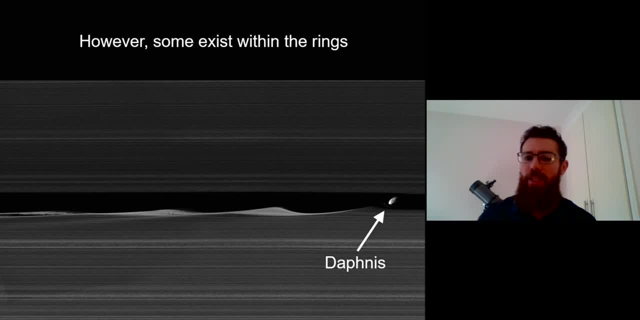 It's inside this very small gap. So what happens there is, the moon is actually creating that gap as it orbits around inside the ring, And that gap is actually related to how big it is as well. This is quite a nice close up image taken by Daphnis. 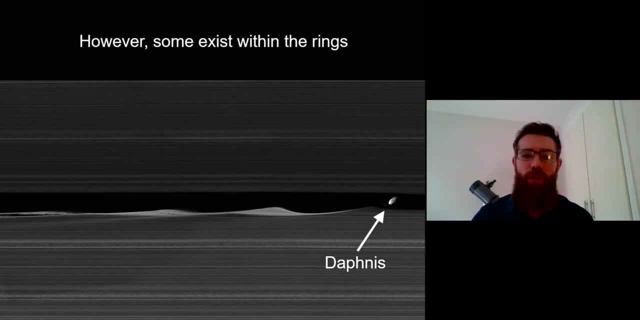 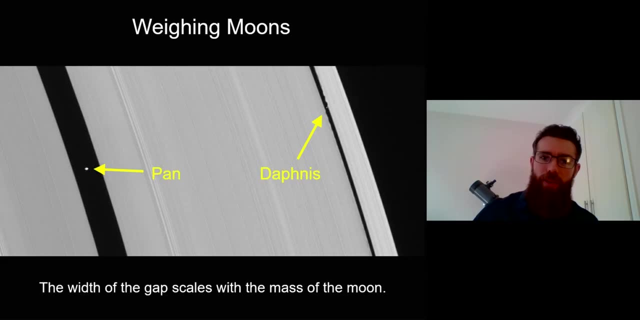 And you can see the wave structure on the edge of the ring as well that that moon is gravitationally causing as it orbits around. But the interesting thing about these moons that are inside the rings is that you can use the gap to weigh the moon. 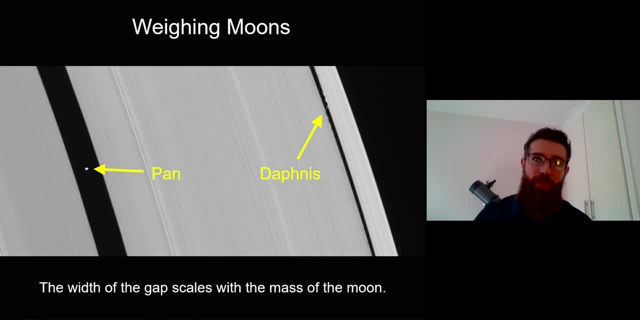 So we have a spacecraft there, We can actually look. Well, we did have a spacecraft there. We can now look at the moons. But if we couldn't see the moons, we could still work out the size of those moons by how wide. 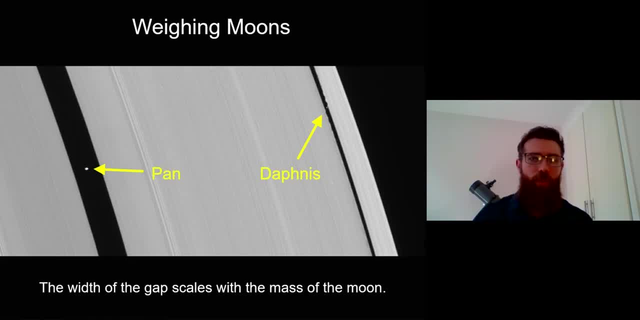 That particular gap was. So you've got these two moons here, Got Pan on the left and Daphnis on the right. Pan is much bigger And, as you can see, it creates a lot wider gap there And we can just use some fairly simple mathematics to work out the width of that gap and the moon that must have actually caused it. 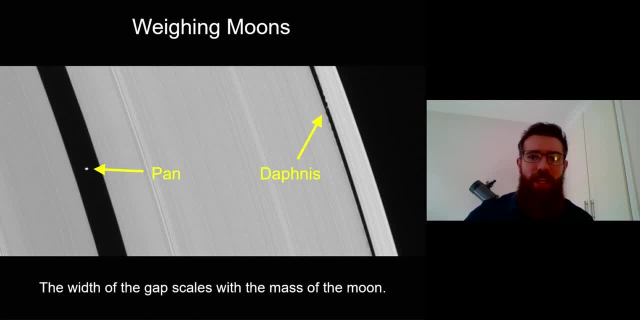 It's quite useful actually, because we can use it to look at rings around exoplanets that we actually can't see in that great detail, But we might be able to work out there's a gap. I mean, you know, if we're doing so, we might also be able to infer the size of a moon we can't actually see. 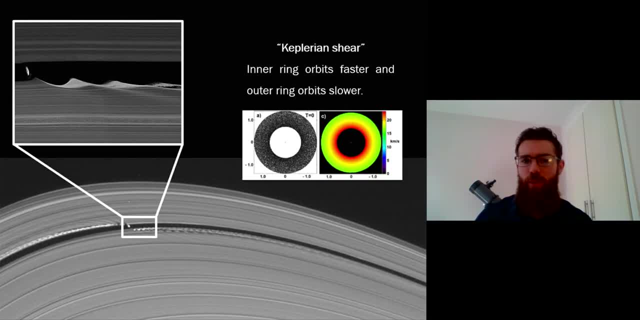 So you can probably see that the waves caused on the ring by this particular moon they kind of offset or they're in different directions And if you remember, from our other short video on planetary rings, we have this Keplerian shear. So it means that any ring particles closer to the planet are orbiting faster than those further away. 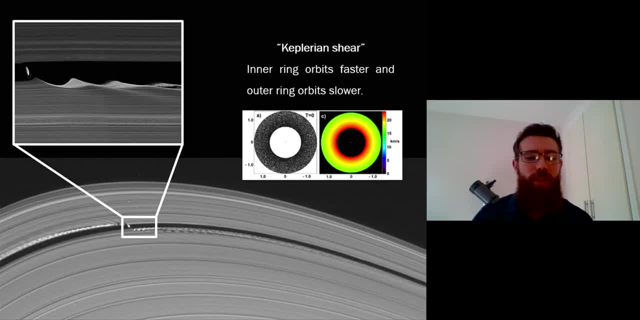 As you can see by the kind of illustration on the right. what that means is that, as this moon is wandering around in the gap, it's causing these waves on the edge of the ring, on the actual gap itself. So it's pulling it around, it's making these waves. 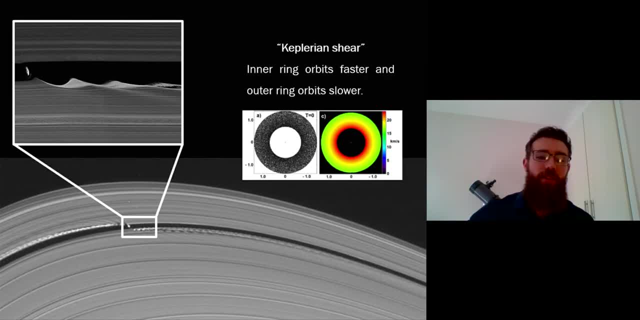 But because the inside of the ring is orbiting faster than the outside, the waves are actually kind of going away, or, in front of it, of the moon as it orbits, and on the outside they're traveling slower, So actually they're downstream. 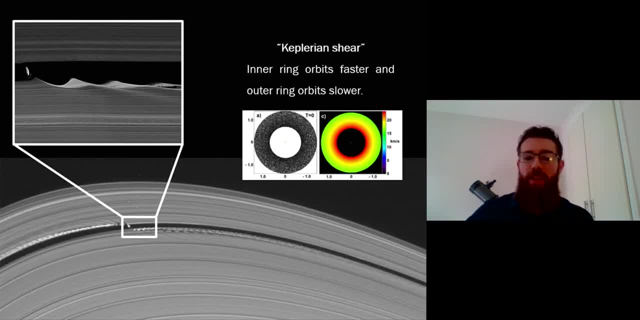 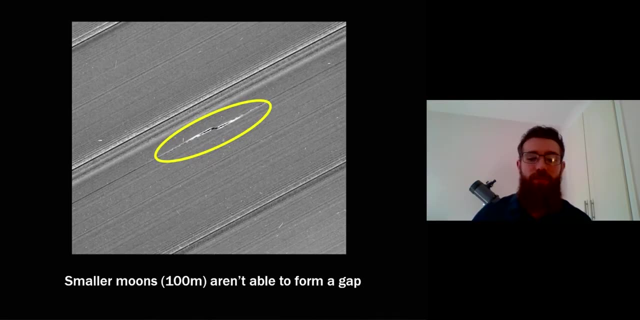 So it causes this kind of structure where closest to the planet they're in front of it and further away they're kind of behind the moon as it's on its orbit. Now, if the moons themselves are not big enough, they won't actually cause a gap in the ring. 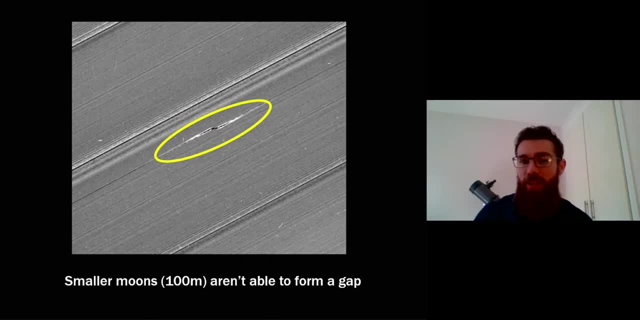 So instead they cause what we would call a propeller shape, And you can see a really nice one here, And it's the same idea with the moons causing those waves. Keplerian shear means that you have one structure kind of one direction and the other structure kind of tailing it behind in the other direction. really. 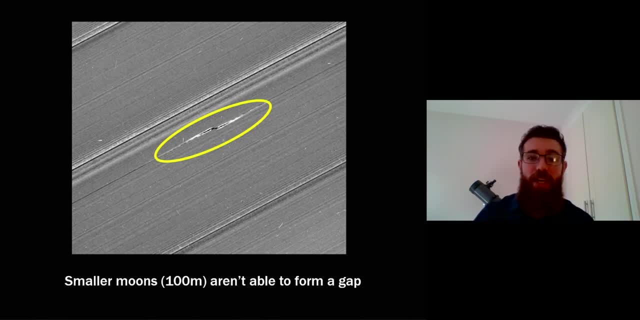 But when they're very small they just don't have enough mass or gravitational influence on the nearby ring to clear it out, So they just distort it locally And we wouldn't necessarily call these moons. Maybe they would be called a moonlet instead. 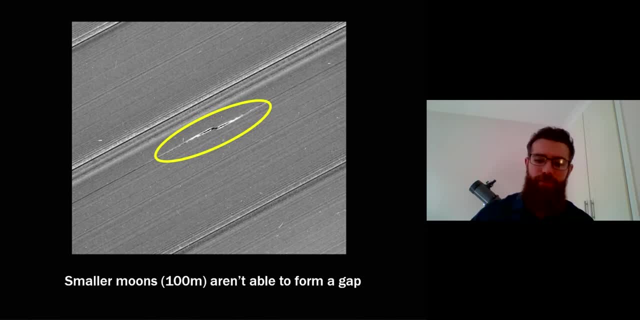 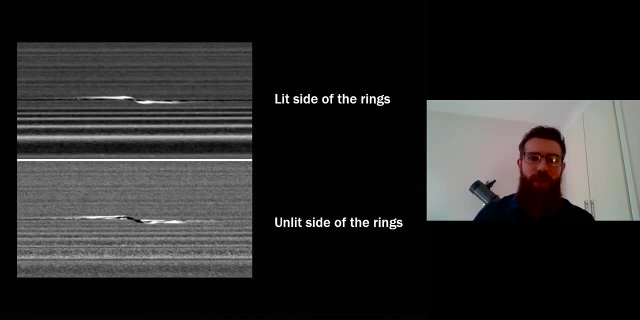 So, instead of a gap, you get this propeller like structure instead, And this is taken from Above the ring and below the ring by Cassini And you can see you've got a really nice propeller shape there And again we might not be able to actually see the moon or the moon that's causing that, because it's so small. 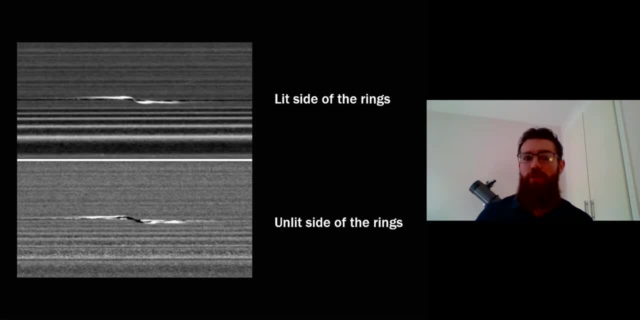 What we can do is look at the shape and size of the structure it's caused on the ring, And then we can probably work out how big that particular object is, And then, finally, you know, we're going to have a look at the F ring. 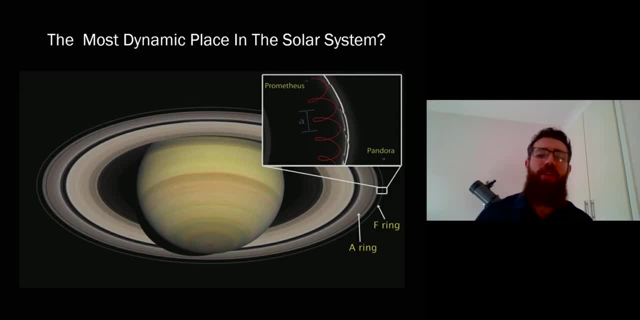 So. So The F ring sits just on the outer edge of the main ring And it's a very interesting place because it's possibly one of the most dynamic places in the solar system. The ring structure changes on a matter of hours. It changes very quickly.